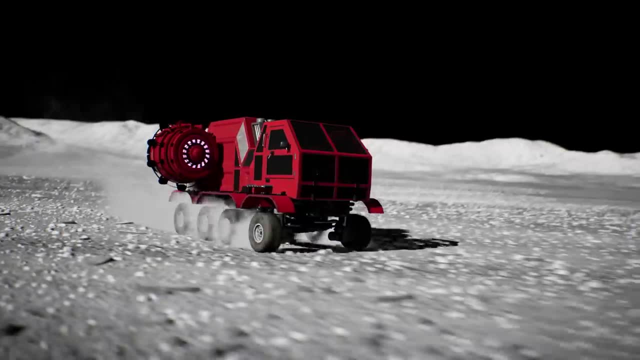 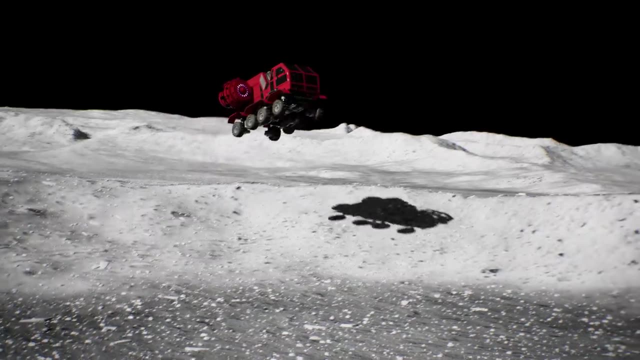 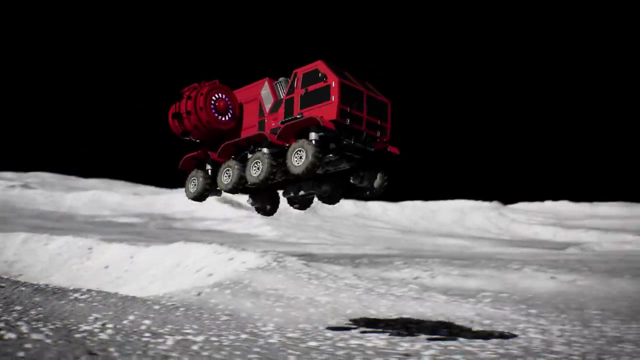 than you could on Earth. And if we drove our space explorer truck on the moon, it could do some amazing jumps, since the moon's gravity is six times weaker than on Earth. Whoa, Look how far that heavy truck can jump on the moon. 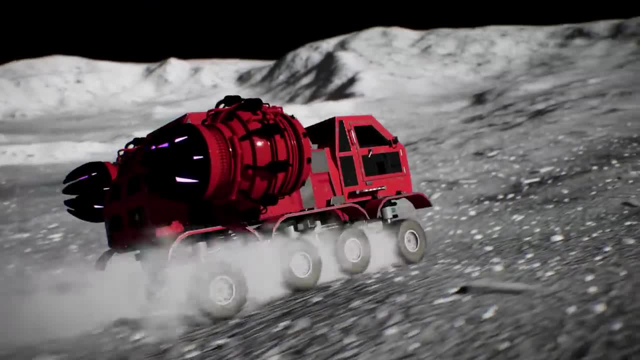 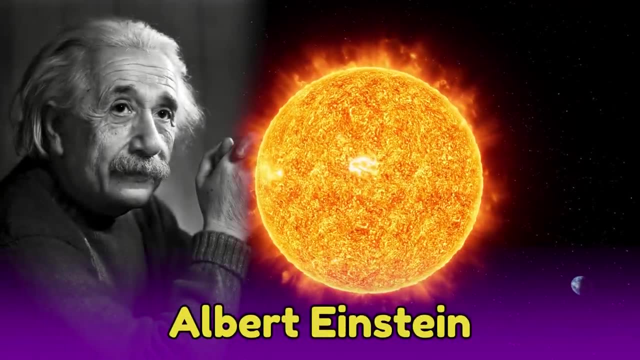 Let's learn more about gravity and how it works. A very smart scientist named Albert Einstein discovered that massive objects like stars and planets will curve the space and make it look like they're in the middle of the moon. And that's how gravity works. 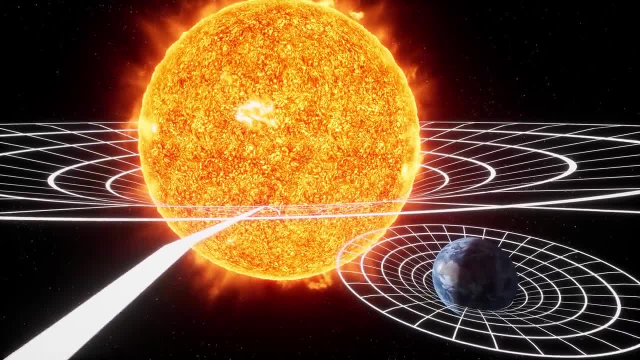 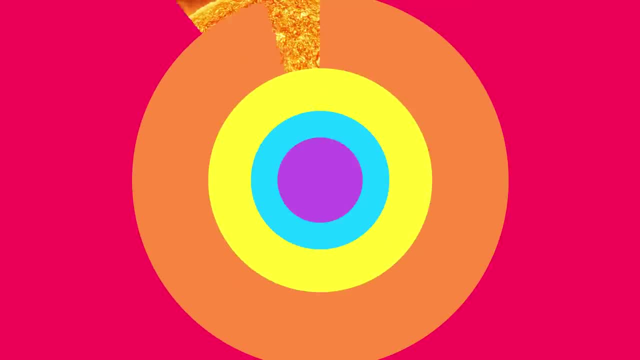 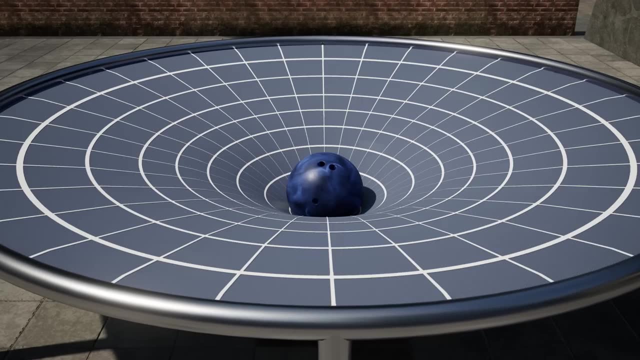 They sort of make a dent in space-time which makes other things fall toward them. It's sort of like if you place a heavy bowling ball on a trampoline, The heavy ball curves the fabric of the trampoline, like a planet will curve the fabric of space-time. 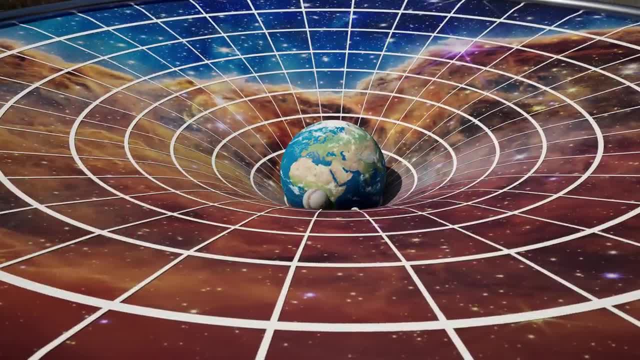 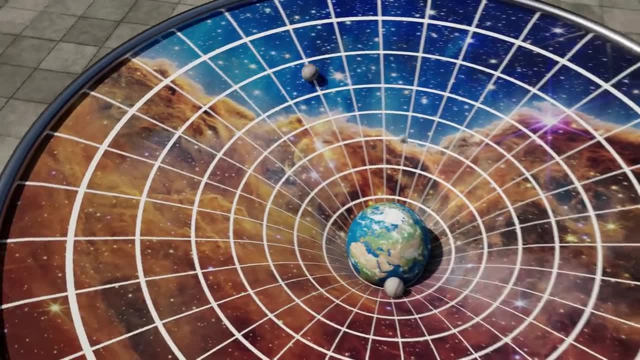 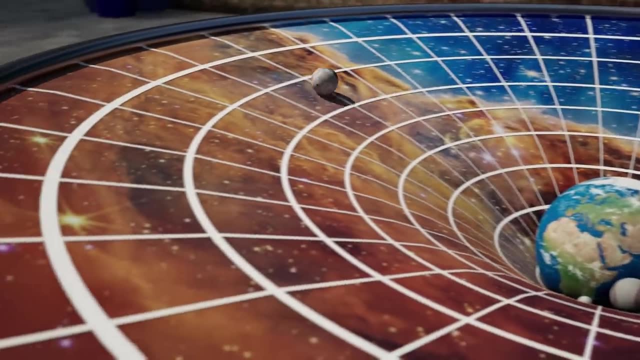 If you place some lighter balls on the curved fabric, they will get pulled toward the heavy object in the center And if you send them rolling around the edge, they will orbit the center almost like how the moon orbits the Earth. Gravity is an important part of how stars and planets move. 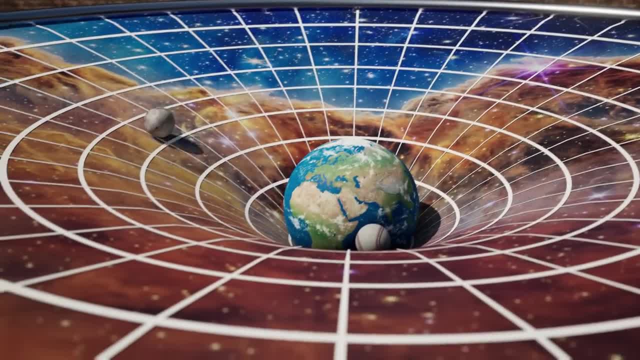 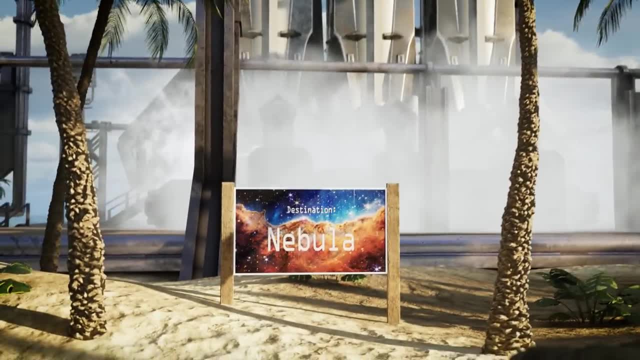 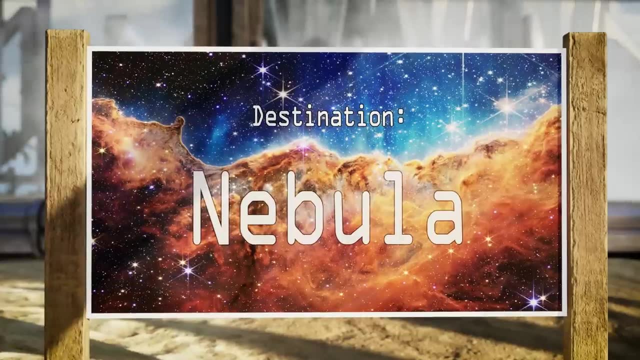 but it's also a key ingredient for how a star is made. OK, let's get ready for our rocket ride into space. We're going to visit a place called a nebula, where we can learn all about how stars are made and how they work. 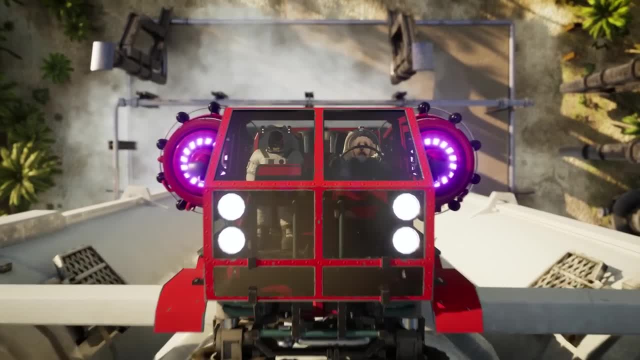 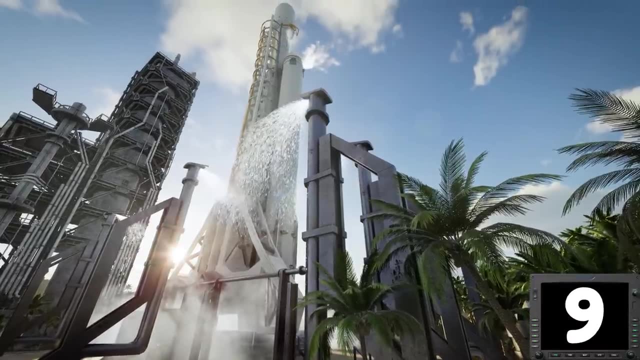 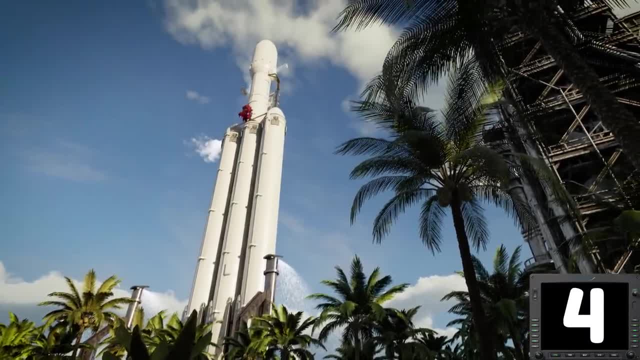 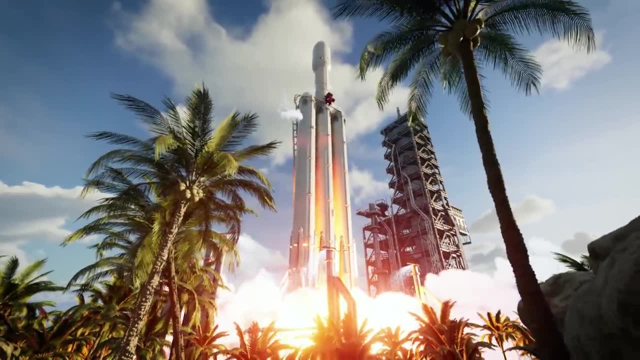 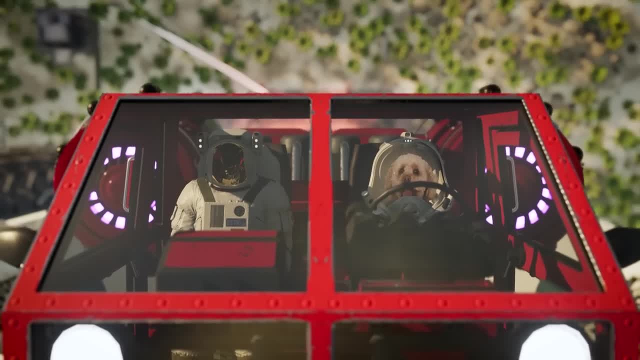 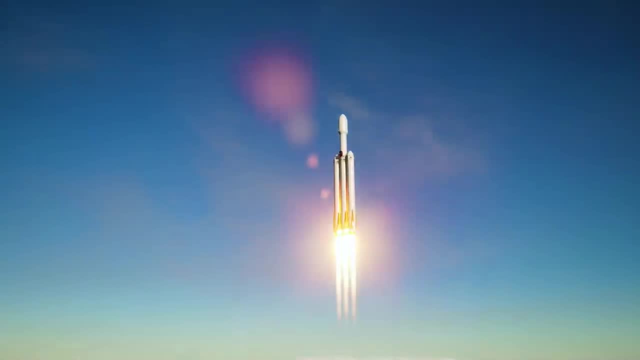 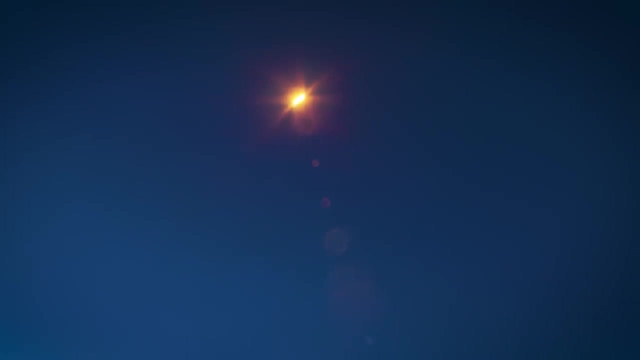 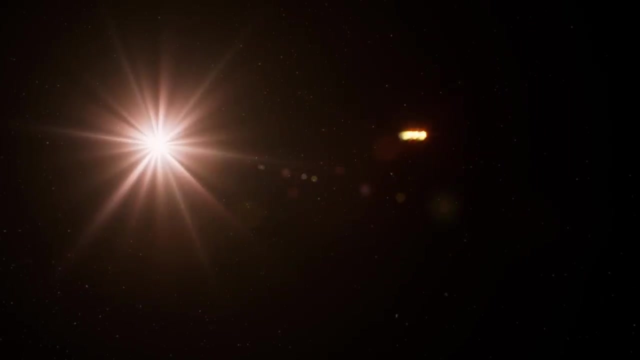 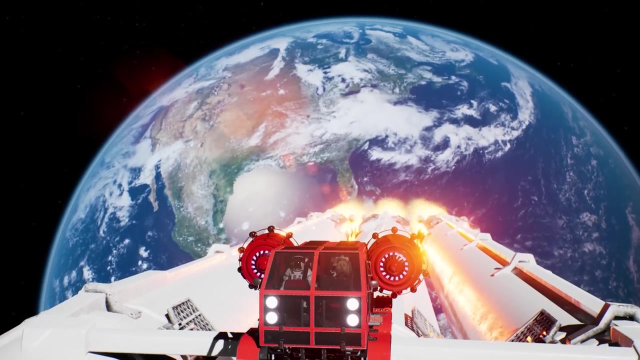 is strong enough to overcome Earth's gravity. Awesome, We made it all the way up into outer space. Our planet Earth looks so beautiful from up here. from up here, OK, Lizzy, time to activate the hyperjets and explore the galaxy. 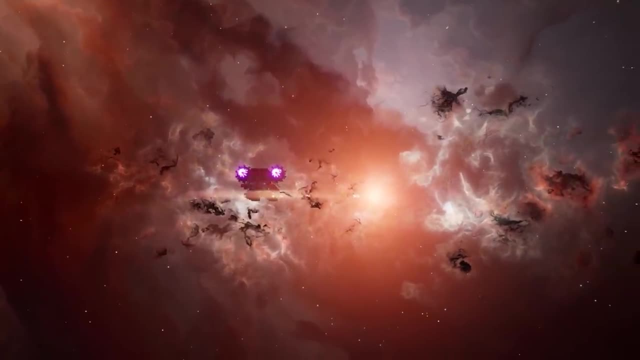 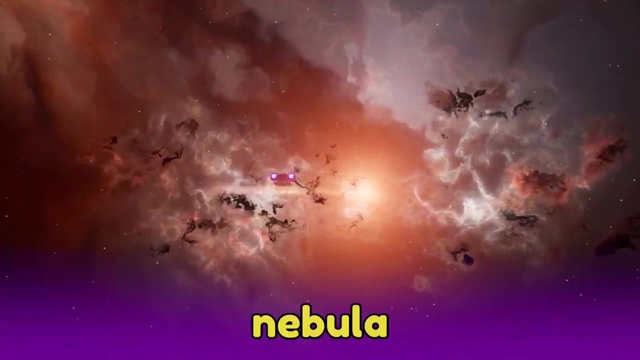 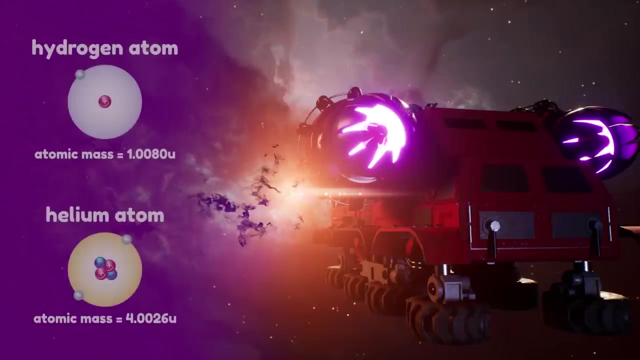 Whoa? look at that. This area of space is called a nebula. A nebula is a huge cloud of dust and gas. They are made mostly of the lightest and simplest forms of matter – hydrogen and helium gas. When these clouds of gas float around in space, 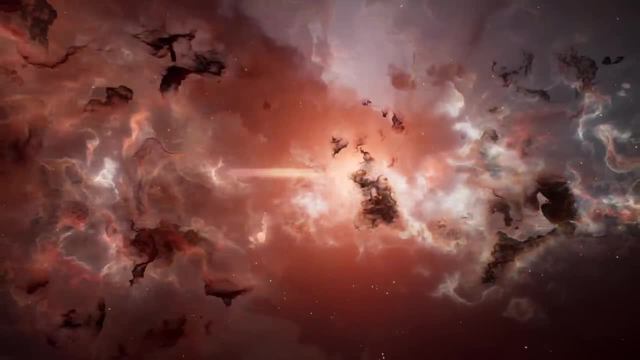 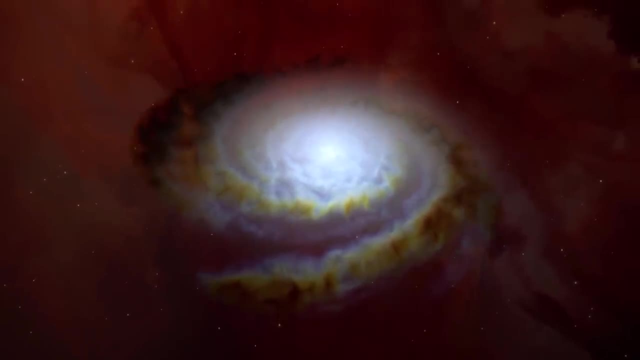 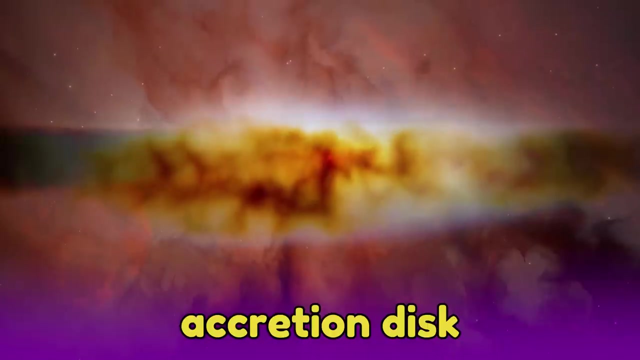 they slowly get pulled together by their own gravity and start to spin. The gas cloud spins faster as more material is pulled into the center and it flattens out into the shape of a disk. This is called an accretion disk. The gas and dust get hotter and hotter. 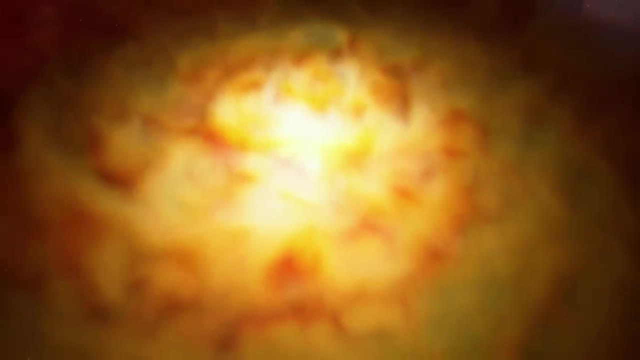 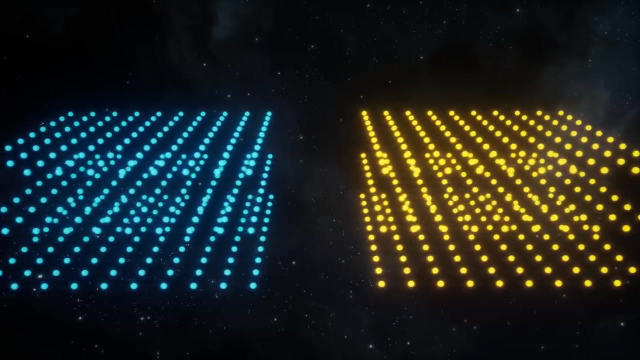 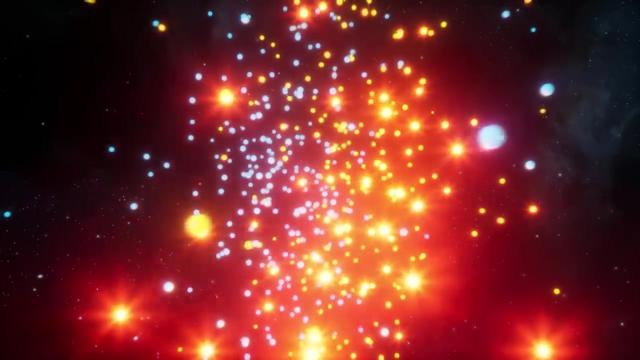 as gravity continues to squeeze it together. Remember when we learned how all matter is made of tiny things called atoms. Atoms have little invisible force fields around them that stop them from getting very close to each other, But in the right conditions they can be made to smash together. 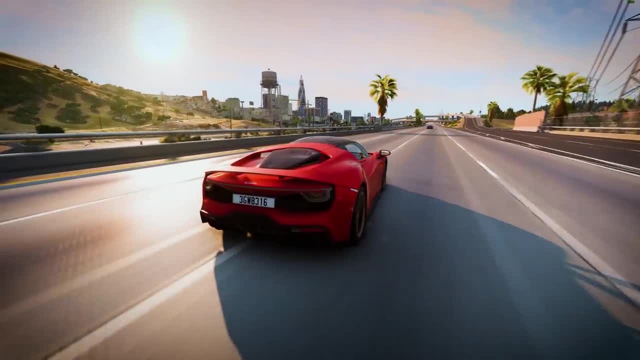 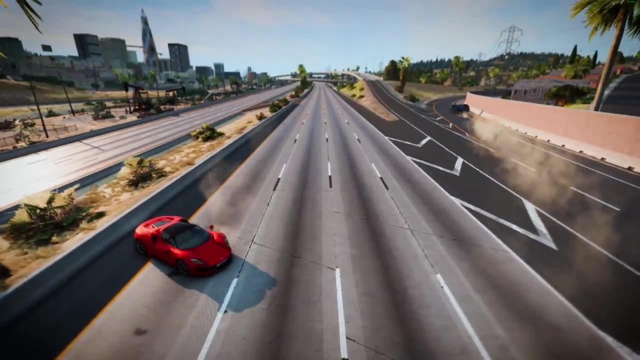 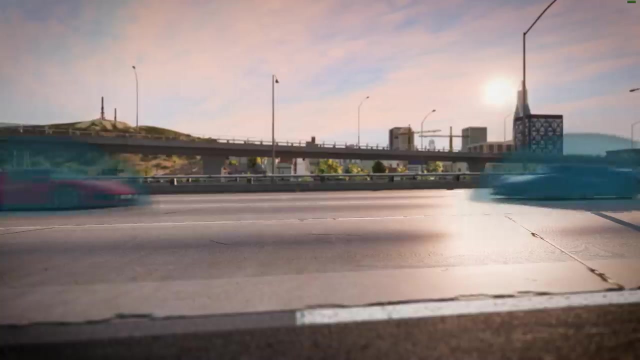 It's sort of like if there are two cars driving down the road with force fields At slow speeds, they will just push each other away when they get close, But if the cars are driving super fast the force fields will not be strong enough. 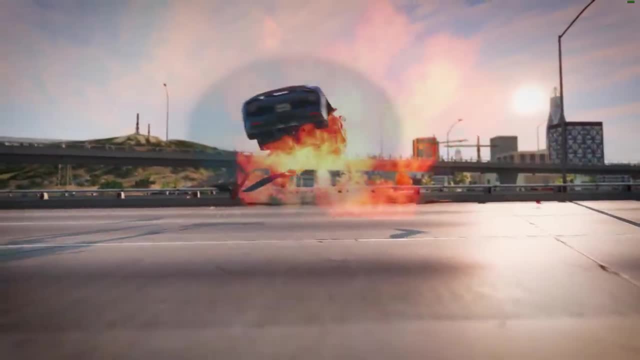 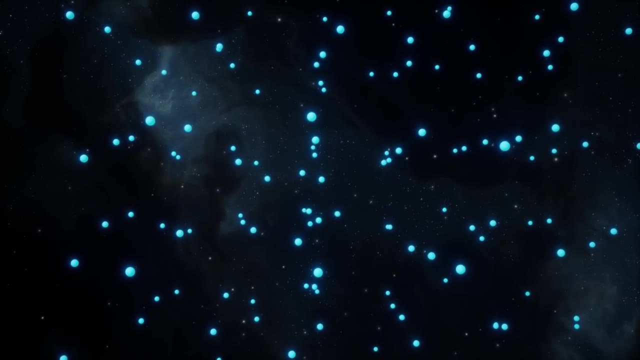 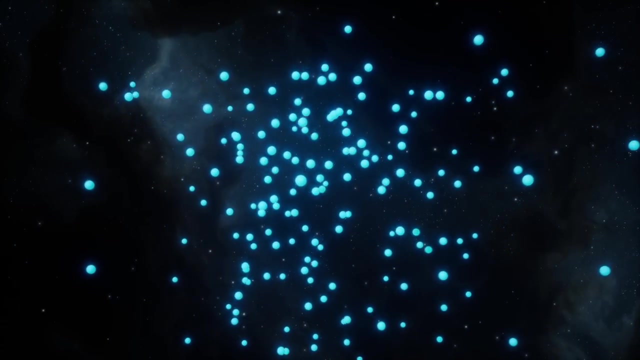 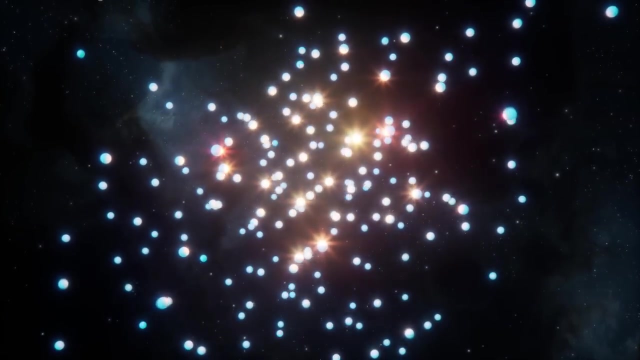 to keep the cars apart and they will slam into each other with incredible force. When gravity squeezes the gas clouds, the atoms will bump into each other, which heats the gas to extreme temperatures and makes the atoms move around super fast. Eventually, the immense heat and pressure 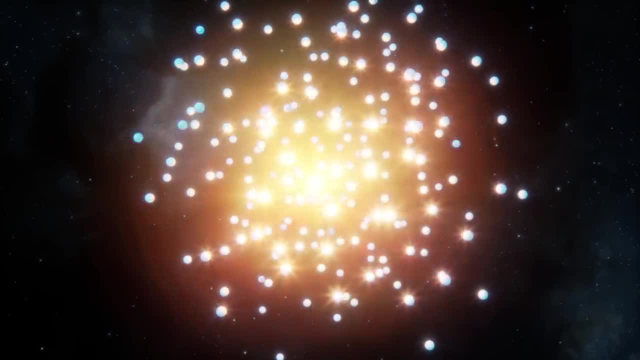 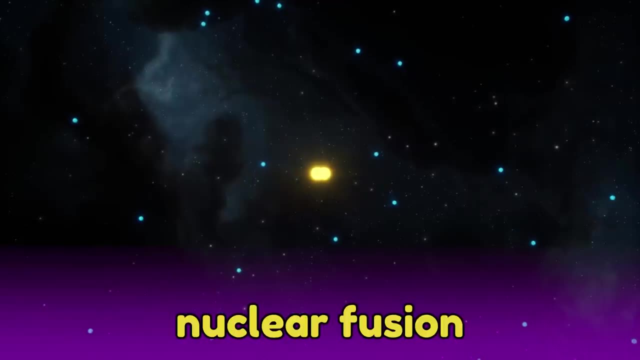 will force two atoms to smash together to make a new, heavier atom. This process is called nuclear fusion and it releases a bunch of energy. This nuclear fusion energy pushes outward and fights against the gravity. The more the gas cloud is squeezed by gravity. 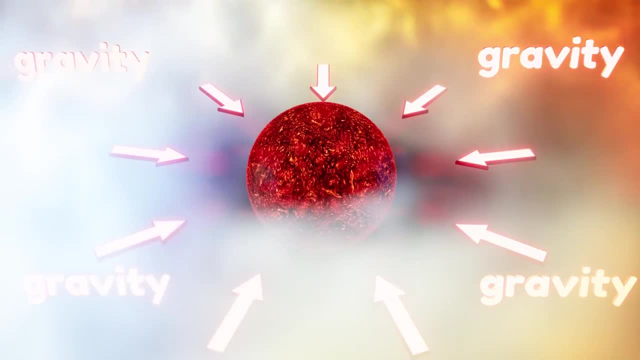 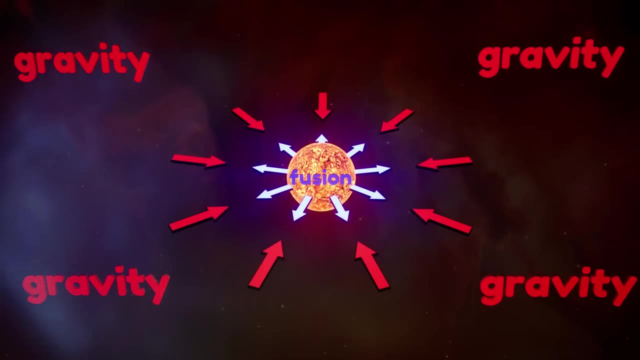 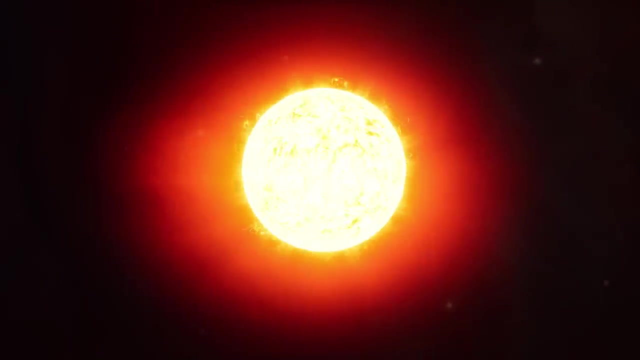 the more nuclear fusion energy is released, until there is enough nuclear fusion to stop gravity from squeezing it any further. When the outward push of nuclear fusion energy equals the inward pull of gravity, it creates a stable star. Hey, this looks kind of familiar. 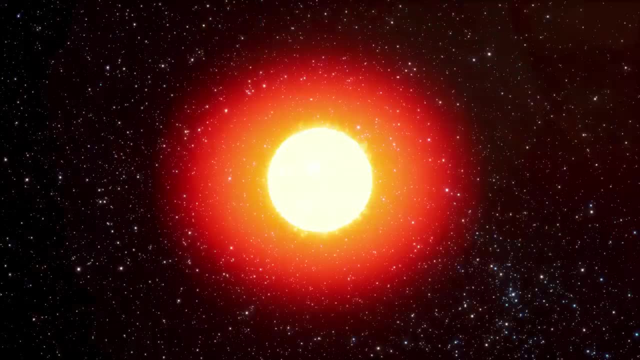 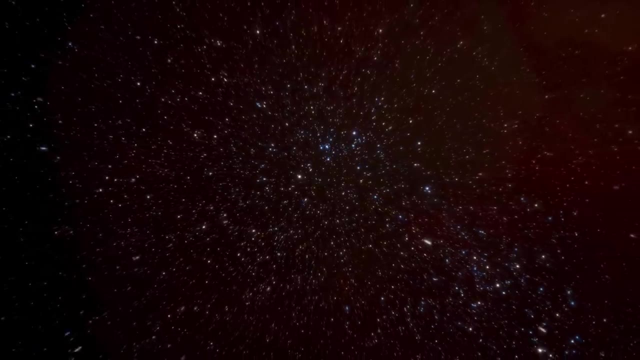 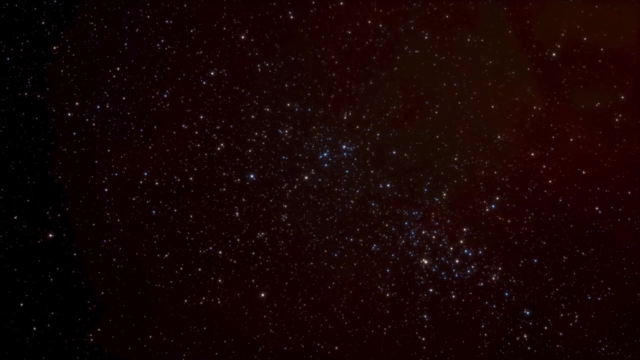 It looks just like the Sun. That's because the Sun is a star, just like the thousands of tiny stars we see in the night sky. It's just way closer to us than any other star, so it looks much bigger and brighter. Our Sun is a medium-sized star. 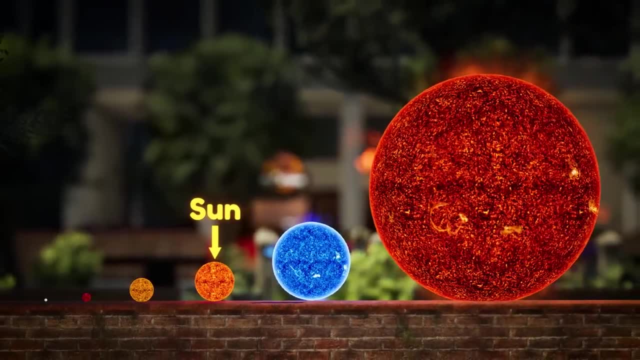 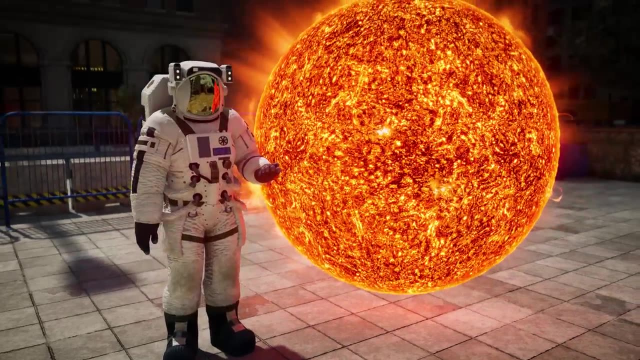 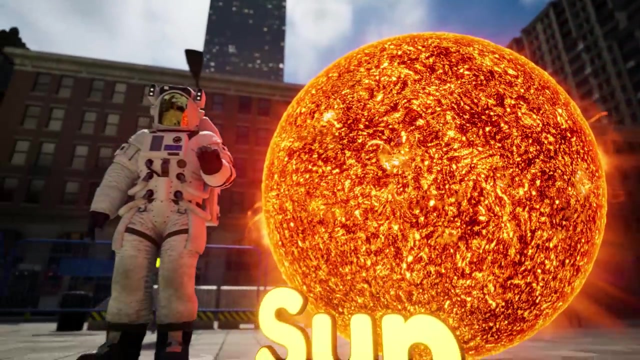 but it's gigantic compared to planet Earth. If Earth was shrunk down to the size of a quarter, the Sun would be 2.6 meters tall. Look how much bigger the Sun is when Earth is placed right next to it. Whoa, the Sun is huge. 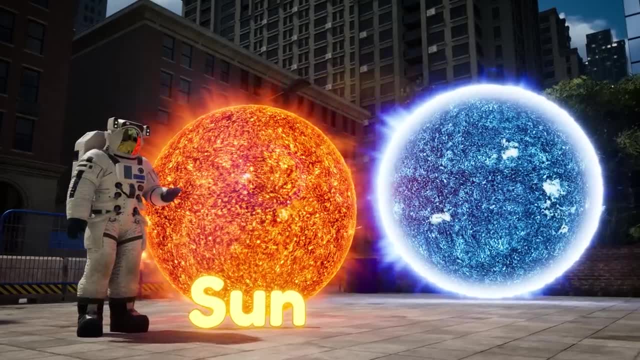 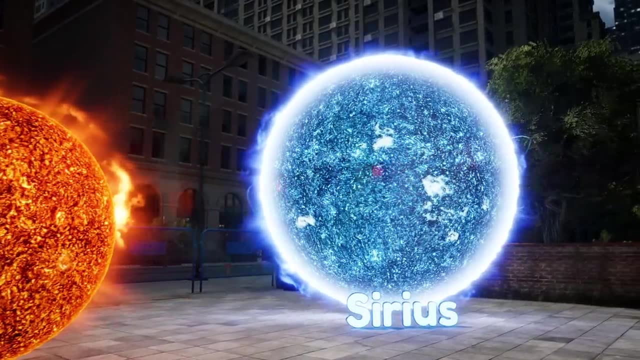 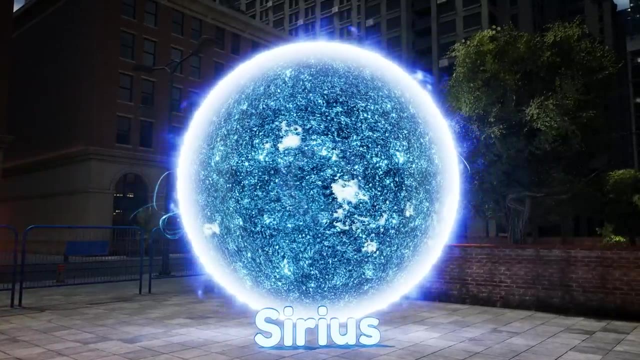 The brightest star in our night sky after the Sun is called Sirius. It burns hotter than the Sun, so it glows a bright blue color, and Sirius is about 1.7 times as big as the Sun. But these medium-sized stars are tiny. 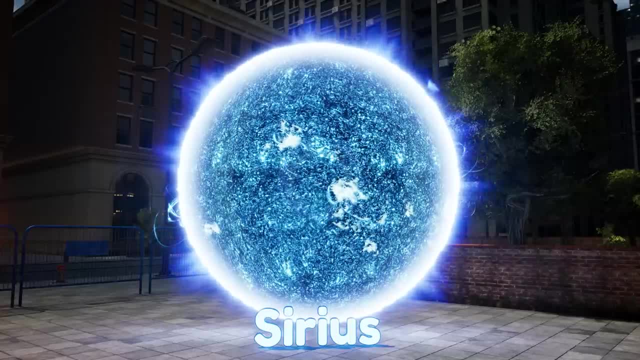 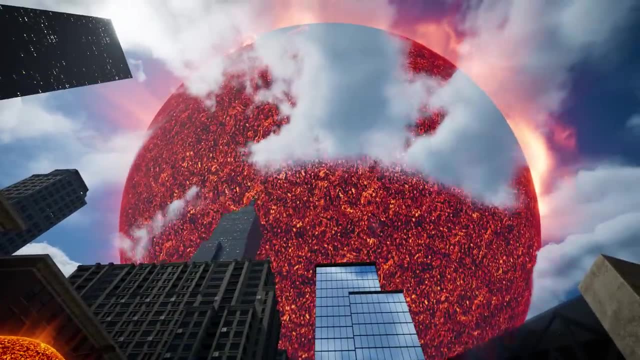 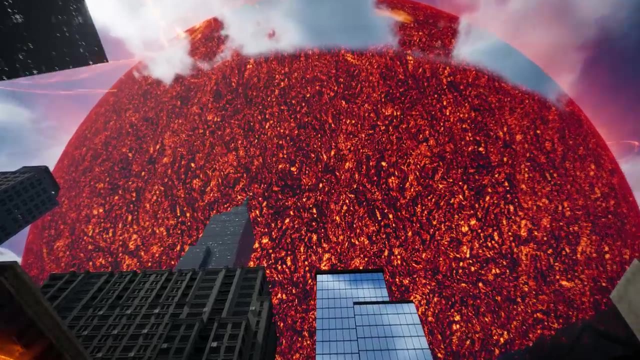 compared to the largest stars in the Universe called hypergiant stars. One of these hypergiant stars is called UY Scuti and it's estimated to be 1,700 times bigger than the Sun. I've placed a scale model of our Sun and Earth. 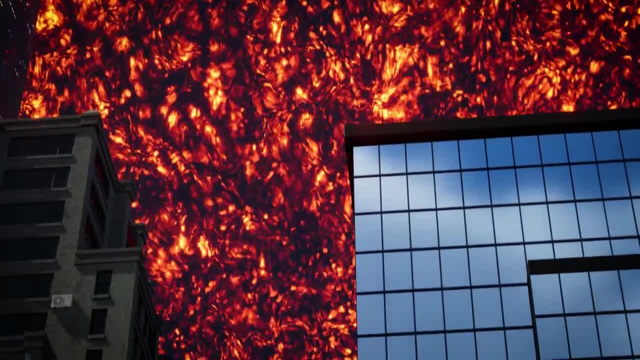 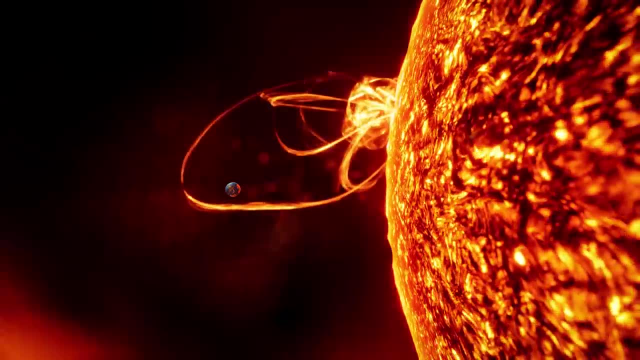 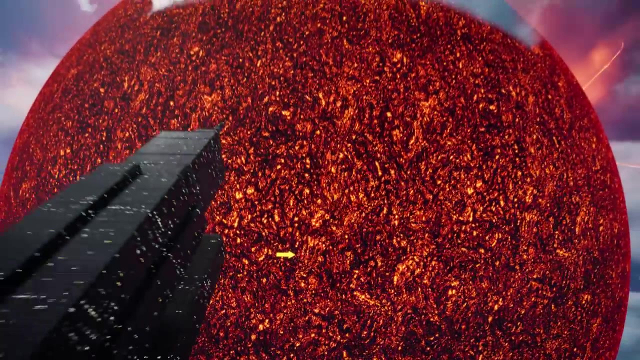 right beside UY Scuti to compare the size. Can you find them? There they are. Let's zoom out to see how big our Earth and Sun are compared to this awesome hypergiant star. Wow, Our planet and Sun are like tiny specks.